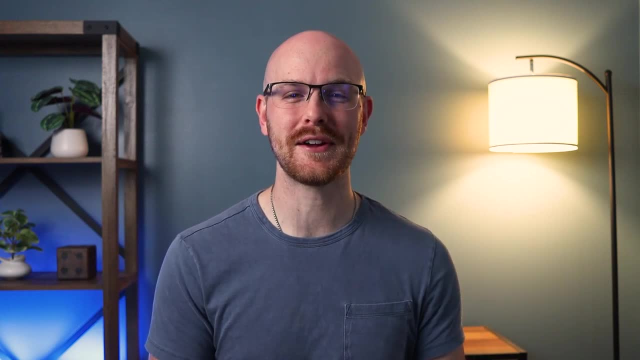 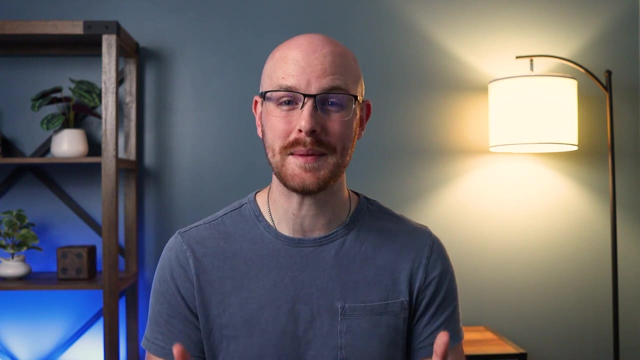 What's going on everybody? Welcome back to another video. Today we're going to be starting our Python web scraping tutorial series. Now, this is more of a continuation of the Python tutorial series, but because we're going to be focusing on web scraping for three or four videos. 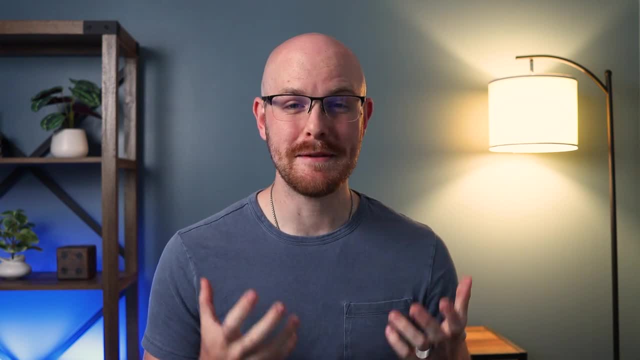 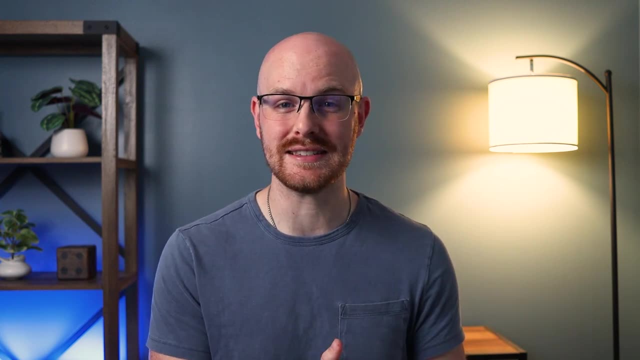 I wanted to just make it its own little mini-series. In this series I'm going to show you the basics of web scraping: how to actually look at HTML, how to inspect a web page, how to pull that data in and then even put it into a CSV file so you can save it and use it Now in this. 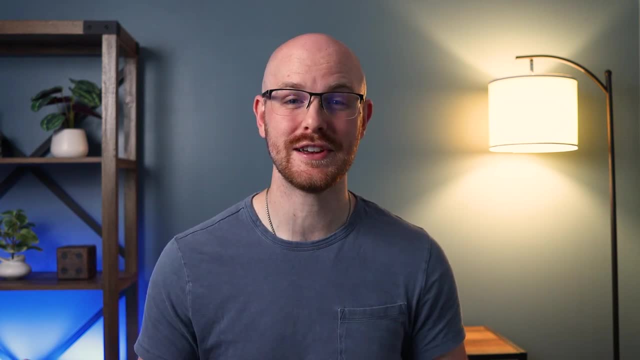 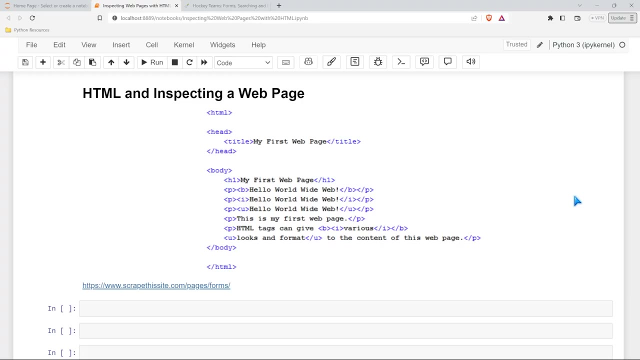 series. we're just covering the basics, which is a fantastic place to start, but in future series I'll be going into some of the more advanced web scraping topics as well. So, without further ado, let's jump on my screen and get started with web scraping Now. the first thing that we need to 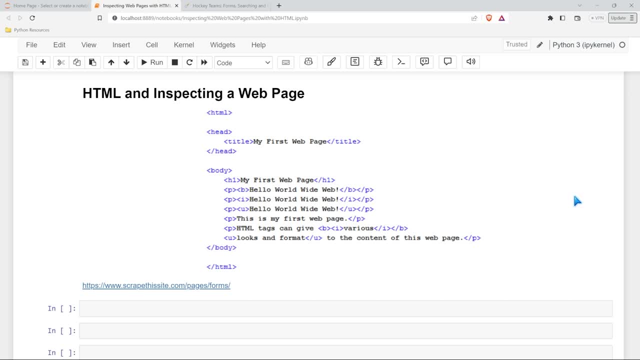 learn is HTML. HTML stands for hypertext markup language and it's used to describe all of the elements on a web page. Now, when we actually go to a website and start pulling data and information, we need to know HTML so we can specify exactly what we want to take off of that website. So 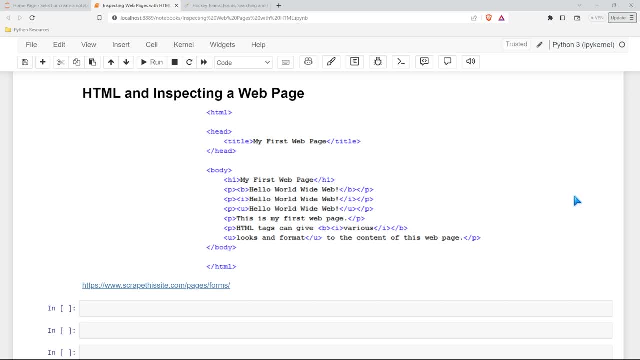